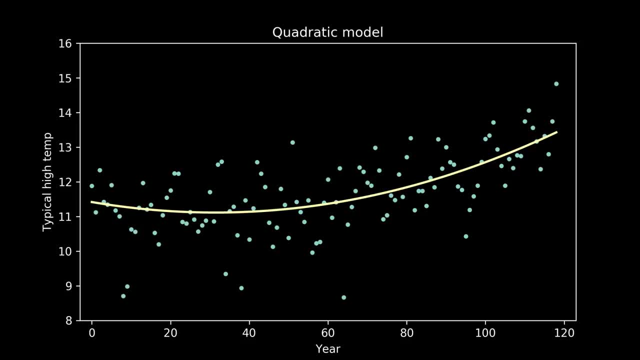 other options. We can try polynomials with cubic terms: powers of three. Or we can look at polynomials with quartic terms: powers of four. We can also fit polynomial models of order. five polynomials of order six. seventh order polynomials: 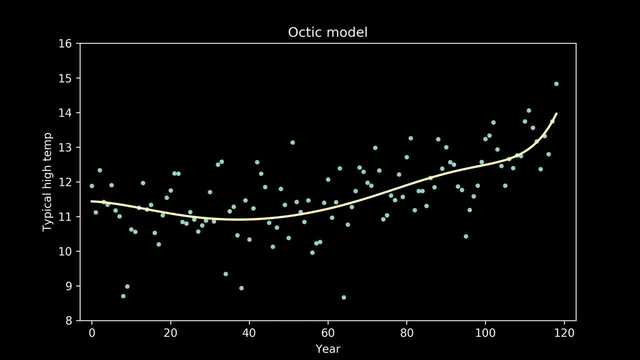 and eighth order polynomials, also called octic polynomials- Useful tidbit for filling lulls in conversations and parties. Now the fit appears to be getting better, But the line is taking on extra personality. It's adopting some wiggles. 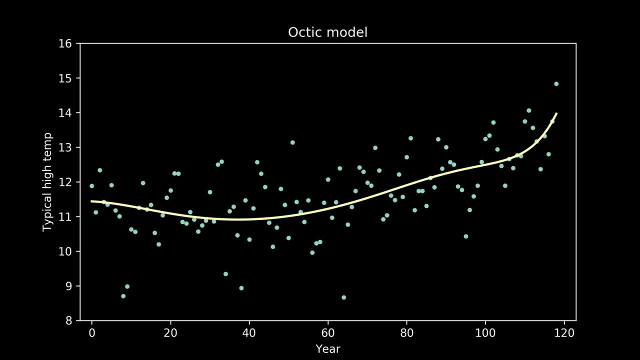 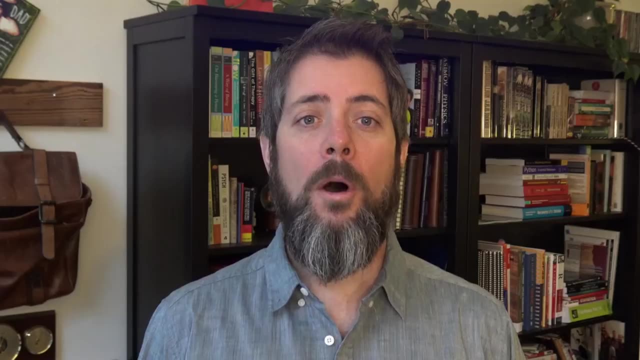 If we take this to an extreme, we can imagine a model that passes through every single data point perfectly. This model would have zero error, zero deviation from our measured data. So does that make it the best fit? model Models are useful Because they allow us to generalize. 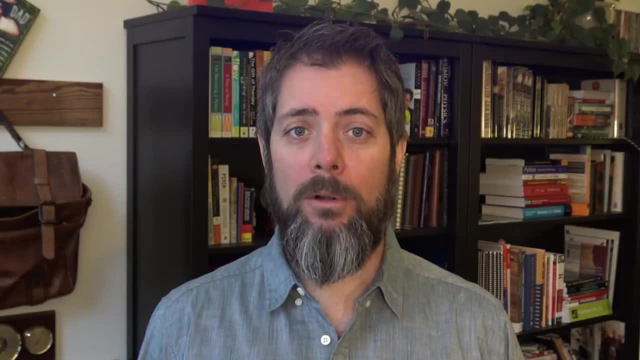 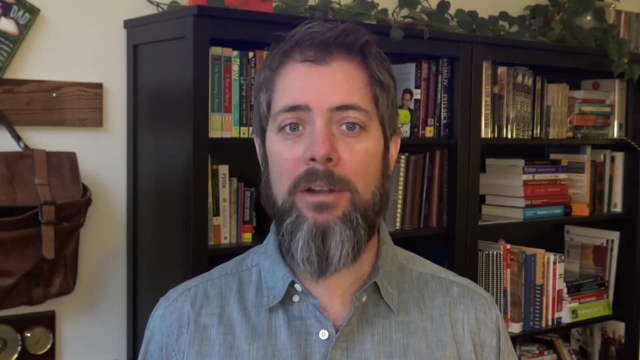 from one situation to another. When we use a model, we're working under the assumption that there is some underlying pattern we want to measure, But it has some error on top of it. The goal of a good model is to look through the error. 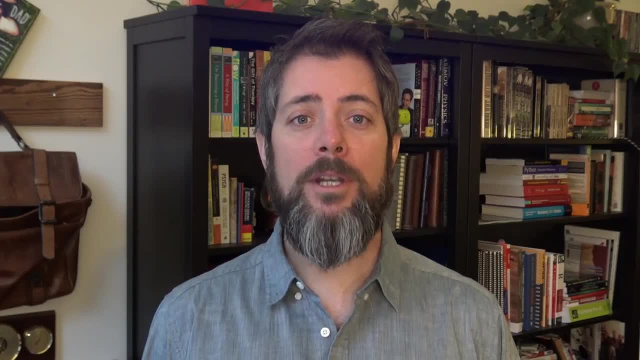 and find the pattern. The most common way to do this is to split our data up into two groups. We can use one group to train our model And then we can test it to see how closely it fits. The first group is the training data set. 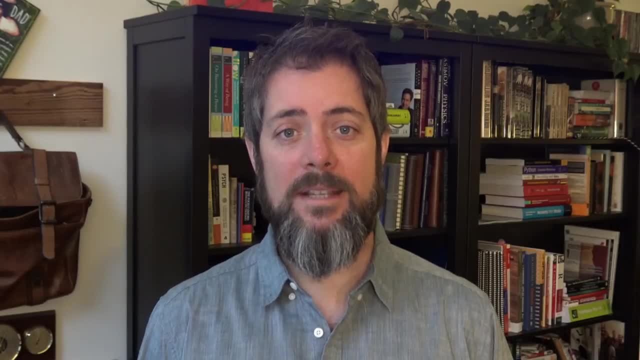 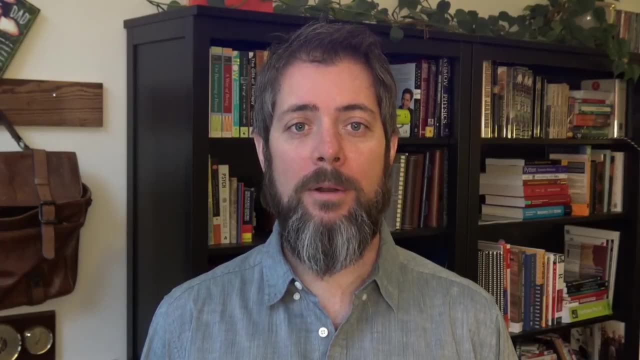 The second group is the testing data set. There are lots of ways to do this And we'll revisit them later, But for now we'll randomly sort out our years into two bins. We'll put 70% of them into the training data set. 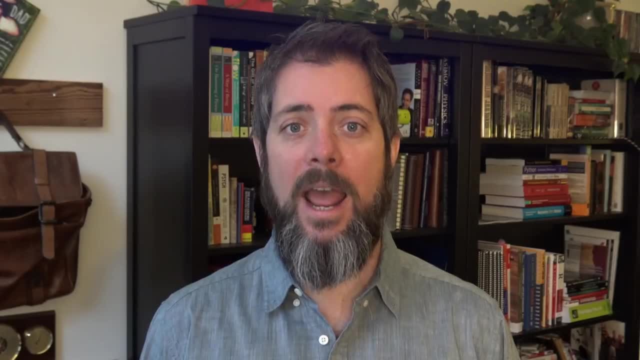 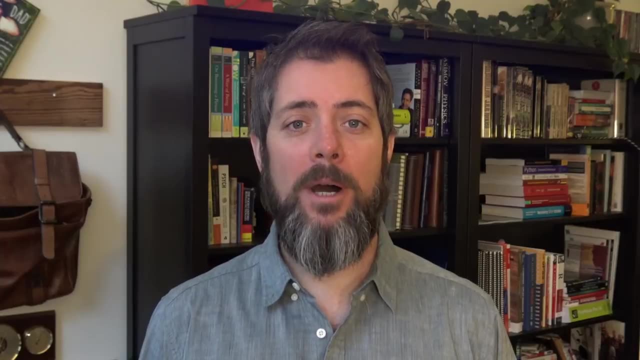 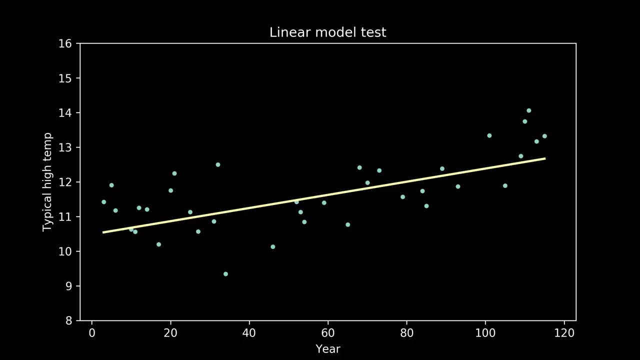 and 30% of them into the testing data set. Then we can go back to our collection of model candidates and try them one by one. Here are a few of our models that we've tested. Here's a sample. Here's a sample of the models trained on the training data. 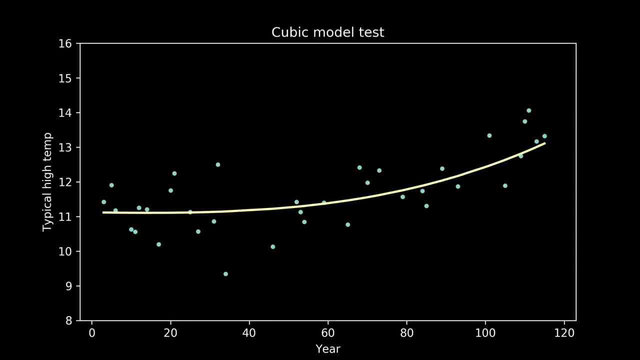 and plotted against the testing data. As the models get to be higher order, we can see that the wiggles they developed may have been helpful for fitting the training data, but don't necessarily help them fit the testing data better. We can see an extreme example of this. 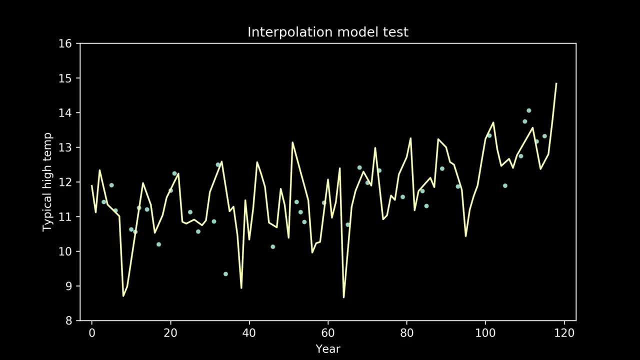 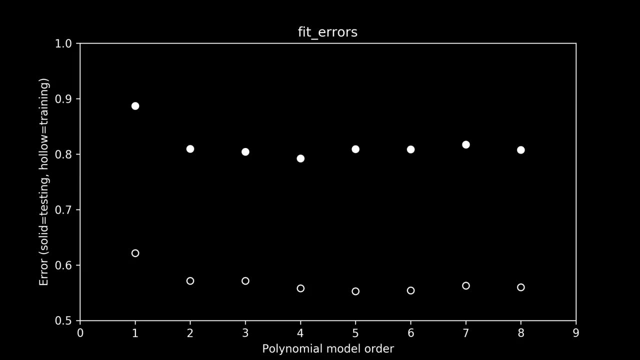 in the full interpolation model where we just connect all the training data points with straight lines, It really struggles to match the testing data points. It's helpful to look at the error on the training and testing data sets for each model, lined up side by side. 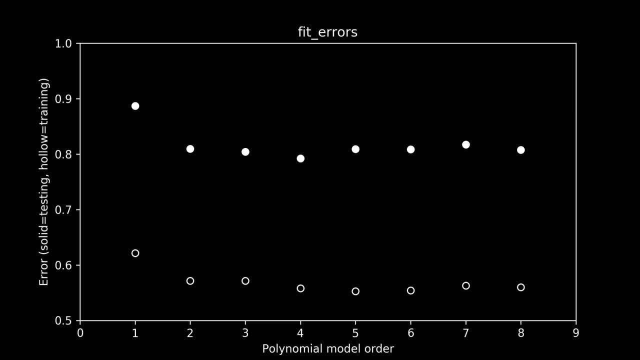 Looking at the errors on the training data set, a few things jump right out. First is the wide gap between the training errors- the hollow circles- and the testing errors- the solid circles. Right away we can see that there's a substantial difference between the two data sets. 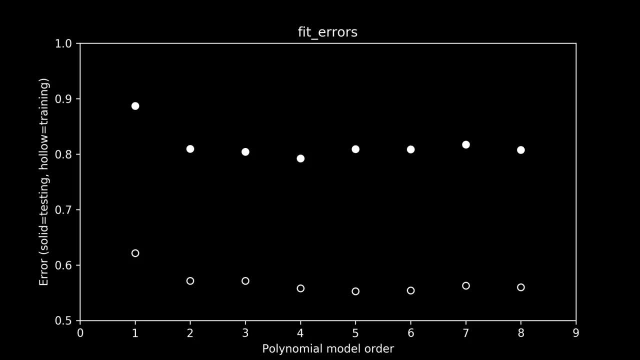 Second, there's a precipitous drop in error going from a linear to a quadratic model. That is a first to a second order polynomial. This makes sense. When we were eyeballing it, we could see that the linear fit failed to capture. 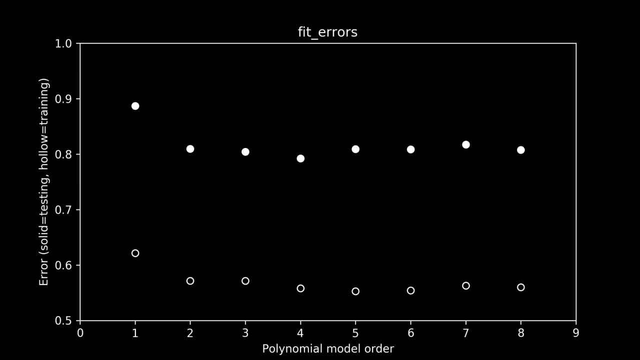 the curvature of the data, one of its most prominent features, The quadratic curve captured that just fine. So which model? Which model fits best? When we look carefully at the errors on the training data, it appears that the error on the fifth order polynomial. 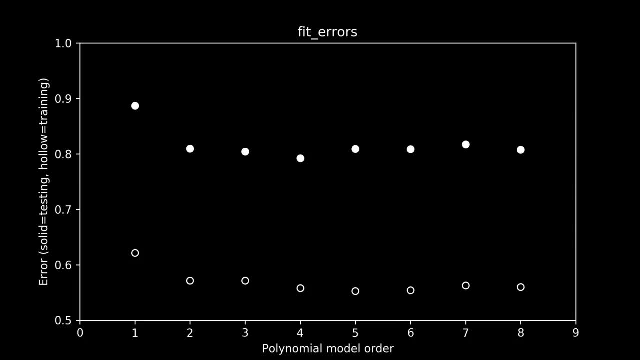 is the lowest. The differences are subtle so you might have to squint, But all the other higher order models have low error too. They're just a little higher than the order five polynomial. But, as we mentioned, that's not the ultimate test. 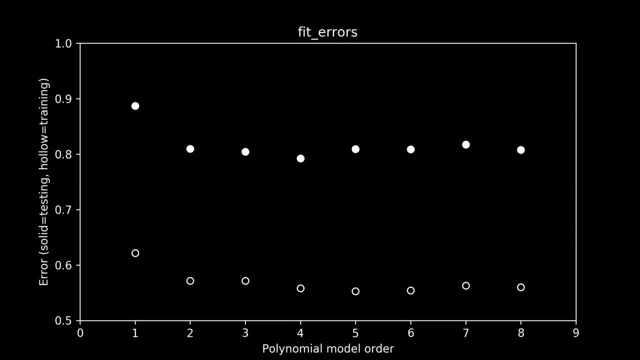 The error on the testing data is what we're going to look at. It's what we really care about. Careful inspection of testing error shows that the fourth order model does the best job At higher orders of polynomials. the error on the test data set. 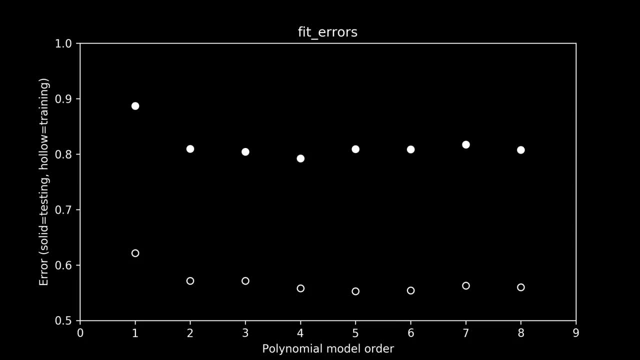 goes up, The more wiggly the line gets in. fifth and higher order polynomial models, the more it captures the quirks of the training data, rather than the underlying pattern of the testing data that we're interested in, Based on this train and test approach. 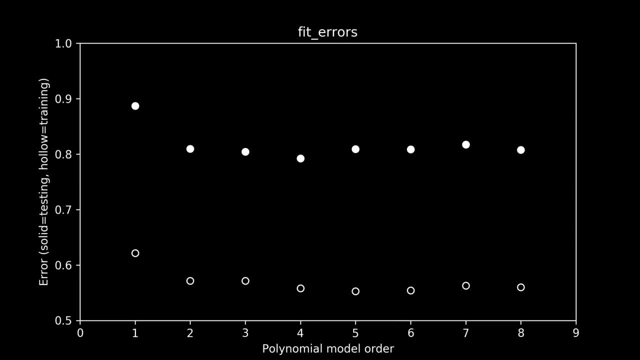 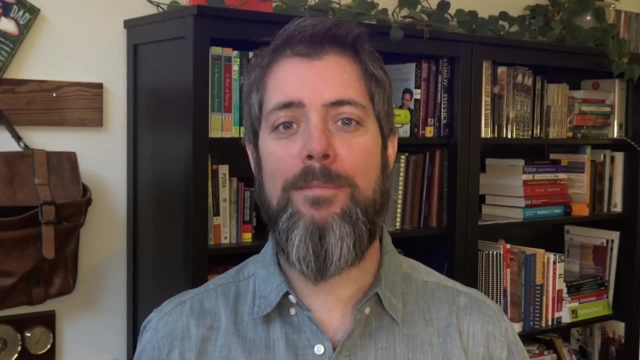 we have a clear winner. Of all the models we tried, the fourth order, polynomial, is best. Congratulations to us. We chose a pretty good model for our data, But don't leave just yet. There are some pretty important ideas still to mention. 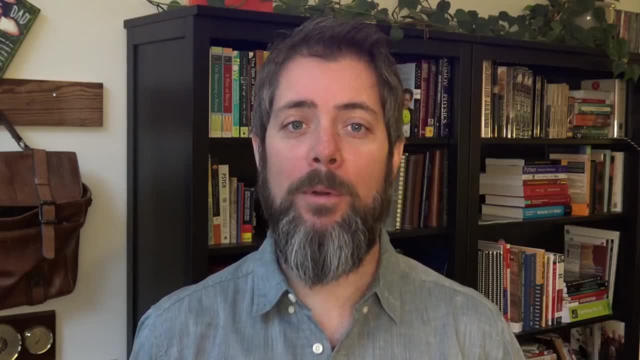 Join me for part two, where we'll talk more in depth about what we want in a model. 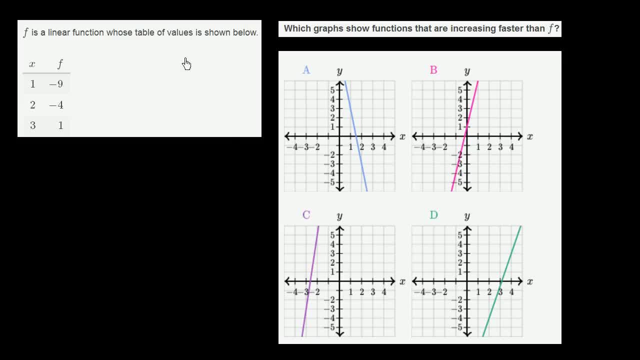 f is a linear function whose table of values is shown below, And they give us three different x values and the corresponding f of x values, Which graphs show functions that are increasing faster than f. So when we're talking about increasing faster, we're really talking about a higher rate of change of y. 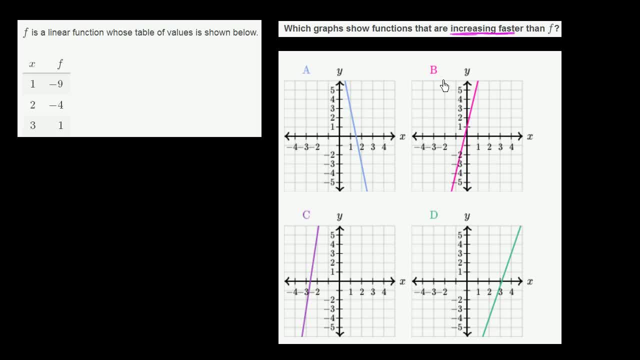 with respect to f, or a higher rate of change of the vertical axis with respect to the horizontal axis, which is another way of saying, is which of these have a steeper slope than the function f? So let's see what the change in our vertical axis. 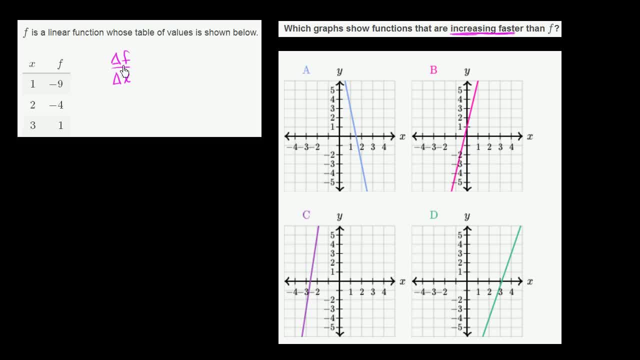 is with respect to our change in our horizontal axis. Once again, the Greek letter, this triangle is the Greek letter delta, which is shorthand for change in. So this is the change in f over the change in x. So we see over here when x changes by 1,. 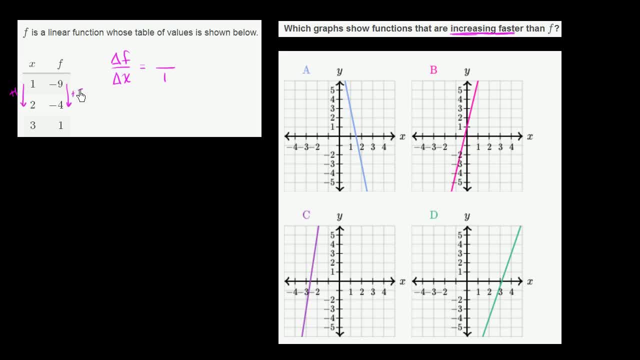 the value of our function changes by positive 5. And it's linear. So that's true between any two points. The ratio between our change in f and our change in x is the same. If we go up 1 again, we have plus 1 in the x direction. 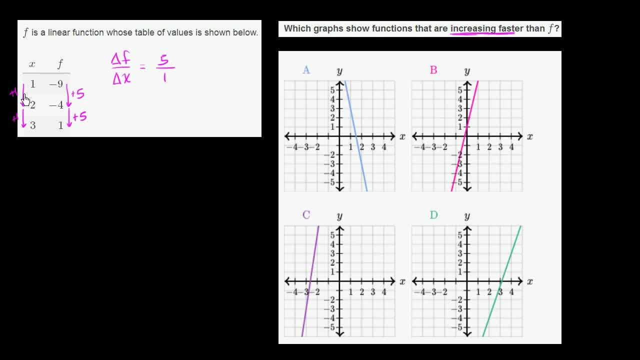 We are once again increasing by 5.. If you start from this point and go all the way here, so if you go plus 2 along x, you're going to go plus 10.. OK, Plus 10 along f, So it would be 10 over 2, which is still 5.. 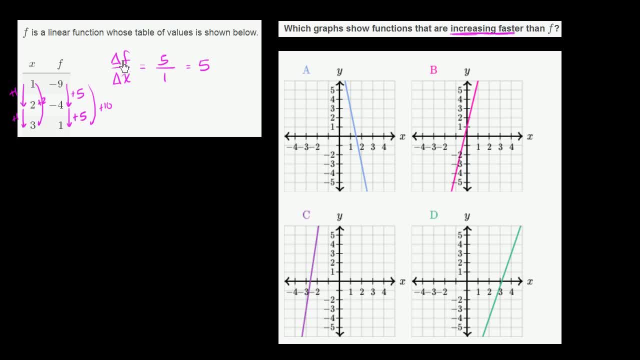 So, either way, the slope or the rate of change of the vertical axis with respect to the horizontal axis is 5 for f. Now let's see which of these increase faster. Well, a, definitely. a isn't even increasing, So we can. a is decreasing.